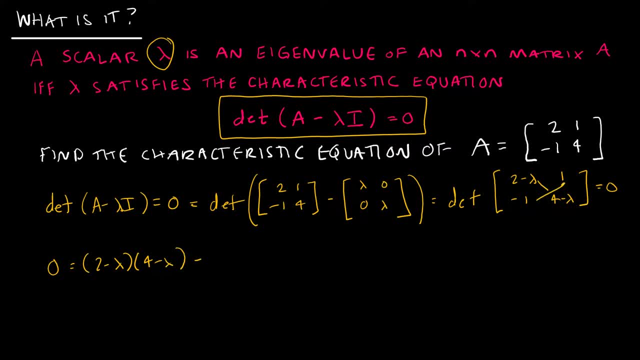 4 minus lambda and I'm going to subtract negative 1 times 1, so that's going to give me 8 minus 6 lambda, plus lambda squared and then plus 1 and that's going to give me, just doing a little rearranging and combining like terms, 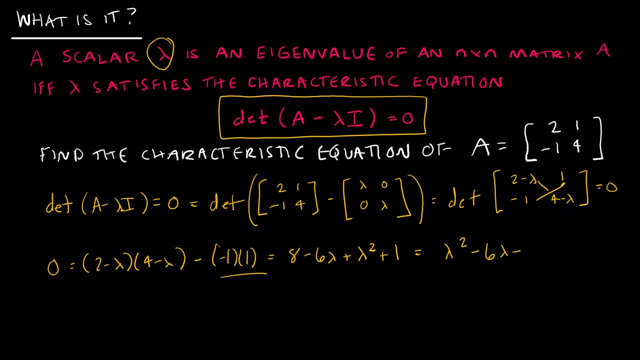 lambda squared minus lambda squared, and then plus 1, and that's going to give me 6 minus 6 lambda plus 9, if we want the characteristic equation. we're going to continue further at this point. what I have is: this is equal to zero, so this is. 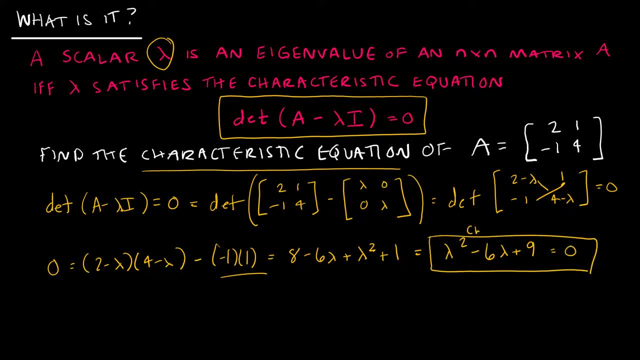 actually called the characteristic polynomial. so when it's all multiplied out, that's the characteristic polynomial. typically they'll make it clear if they want it to be the characteristic polynomial or the characteristic this in factored form or expanded form. If not, it's a safe bet to put it in both forms. 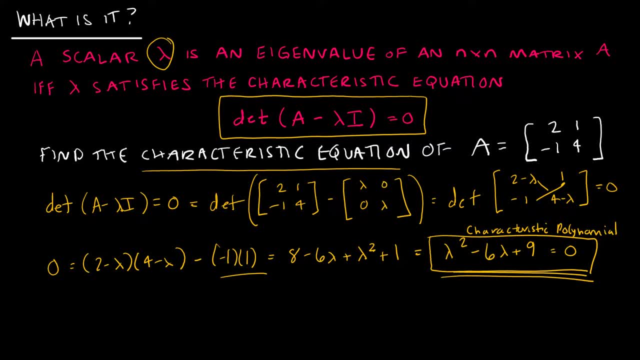 So characteristic polynomial typically means they want you to expand it out. What I'm going to do is then go ahead and find the characteristic equation, which is to go ahead and factor this. So I'm going to say, if I factor lambda squared minus 6, lambda plus 9, that would 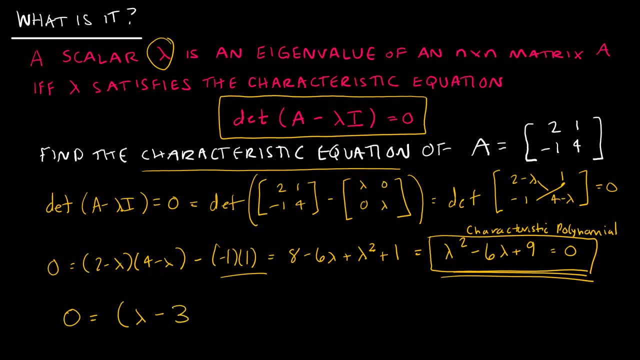 factor into lambda minus 3 quantity squared. So lambda minus 3 quantity squared equals 0, is the characteristic equation. It's very easy at this point, obviously, to then find the scalar or eigenvalue, and I do that then by saying lambda minus 3 must be equal to 0, just like I would if 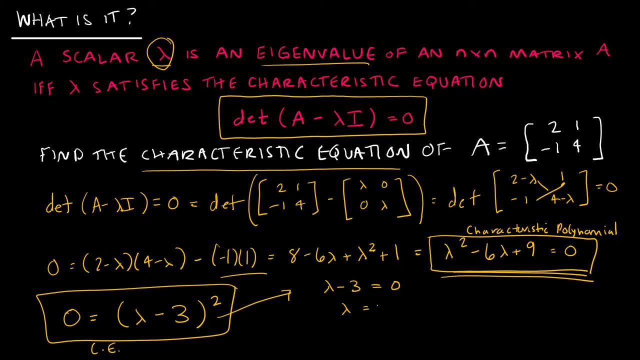 this was a normal polynomial, Which means lambda must be 3.. So 3 is my eigenvalue. 0 equals lambda minus 3. quantity squared is characteristic equation. Characteristic polynomial is typically- they want you to FOIL that out. Let's do a question that has a larger matrix to deal with. but, as we can see, 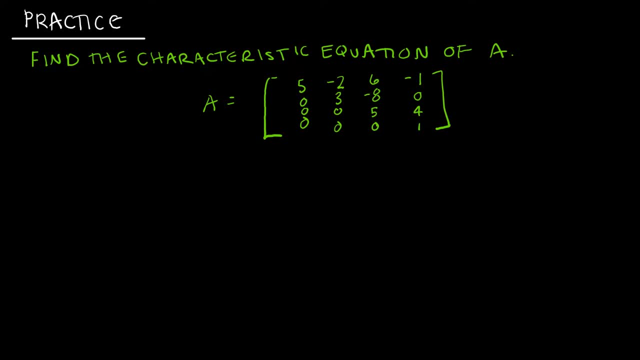 this one is unique because it's already an echelon form, which will save us a little bit of time. I'm going to go about this the same way, So I'm going to subtract: lambda times the identity. so that's lambda. 0 0. 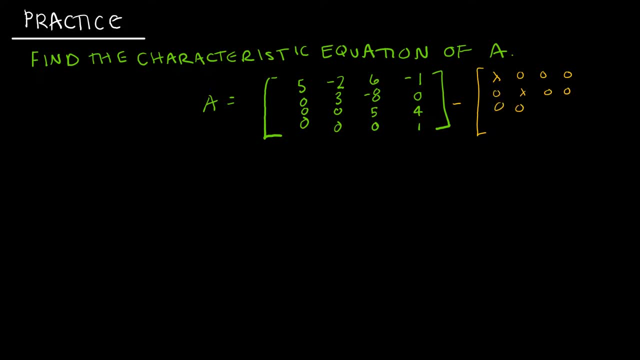 0 0 lambda- 0 0 0 0 lambda- 0 0 0 0 lambda. so, as I'm subtracting this, remember that I'm going to find the determinant of a minus lambda times i, and so that means i'm finding the determinant of. 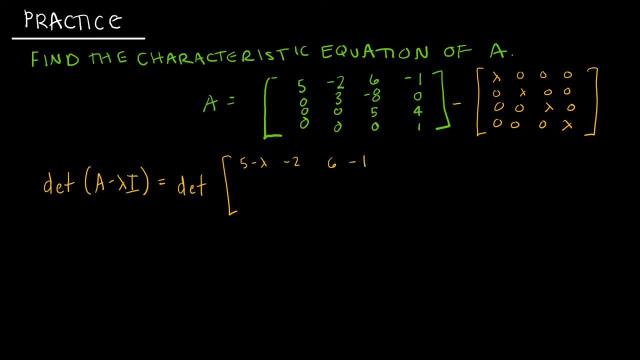 5 minus lambda. negative 2: 6 negative: 1: 1, 0, 3 minus lambda negative 8, 0, 0, 0, 5 minus lambda 4, and 0, 0, 0, 1 minus lambda. 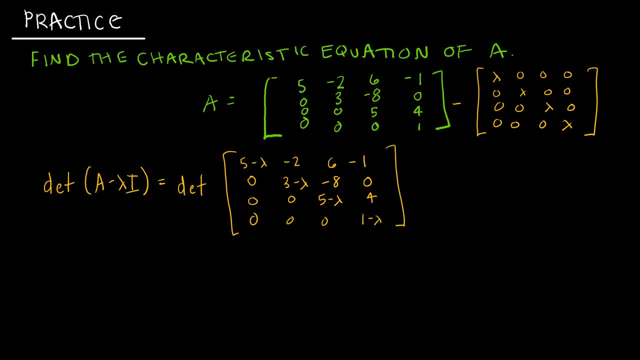 Now, lucky for us, we know that if we have a matrix that is in echelon form- which I do because I've got my nice little zeros here- that in order to find the determinant, all I have to do is take the product of the diagonals. 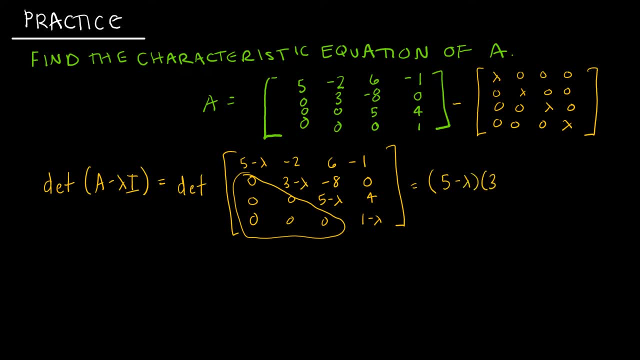 So 5 minus lambda, 3 minus lambda, 5 minus lambda, 1 minus lambda. If they say just find the characteristic equation, then I'm going to say: 0 equals 5 minus lambda, quantity squared: 3 minus lambda. 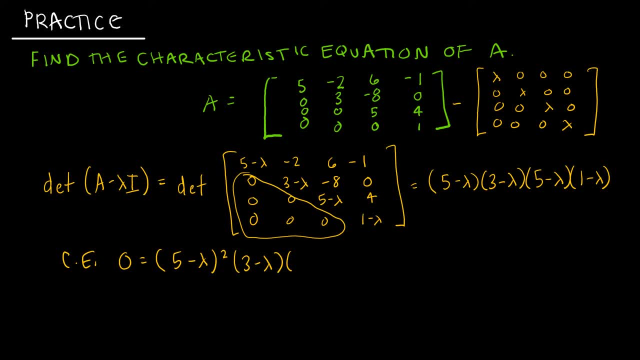 3 minus lambda, 1 minus lambda, If they say to find the eigenvalues, the eigenvalues would be 5, and this one again occurs twice and we just say that has a multiplicity of 2.. 3 minus lambda means I've got a lambda value of 3 or an eigenvalue of 3, and then 1 minus lambda, an eigenvalue of 1.. 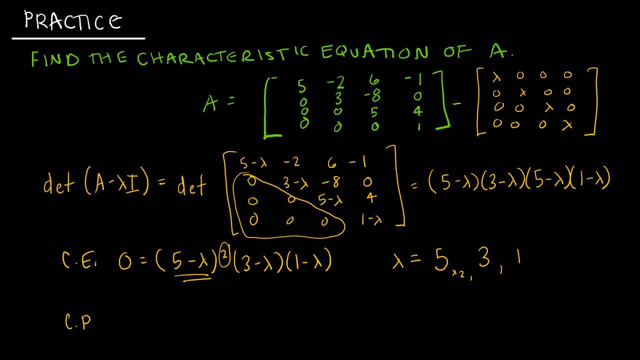 If they wanted me to find the characteristic polynomial. typically that means they want us to multiply that out And that would be: lambda to the 4th minus 14. lambda to the 3rd plus 68. lambda squared minus 130. lambda plus 75.. 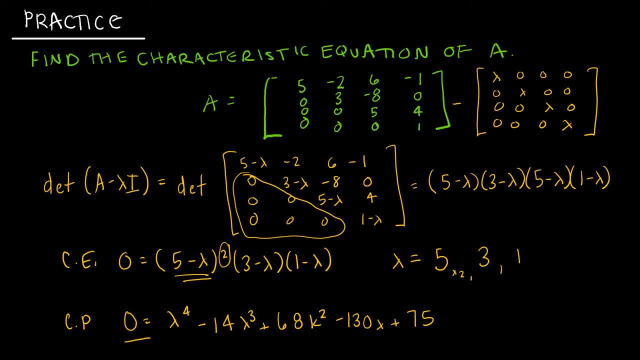 And again, make sure that you have that set equal to 0.. And again, this is a characteristic Equation. this is the characteristic equation. They're both a characteristic polynomial. Just pay attention to instructions. If it specifies expanded form, then you have to do, you have to write it out. 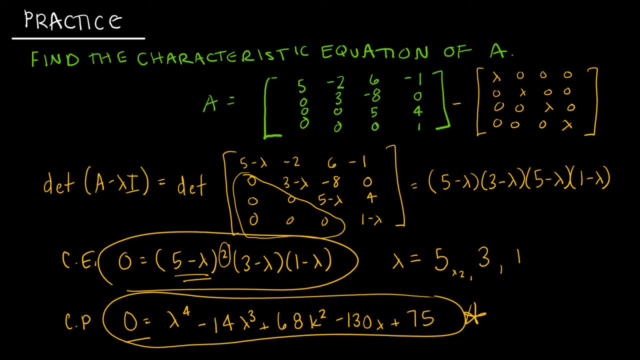 If it just says characteristic polynomial, again not a bad bet to put it in both forms, but this just seems like sort of a waste of time. So for my class specifically, go ahead and just leave that in the factored form. 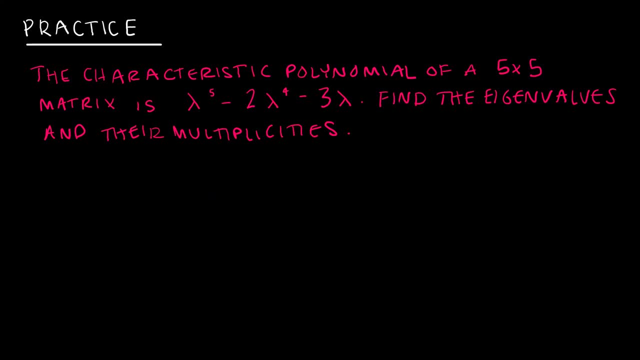 Here's just one more practice for us to do, and if you're feeling up to it, go ahead and press pause and try this one on your own. If not, that's okay, We'll go through it together. So this question gives me a characteristic polynomial for a 5 by 5 matrix. 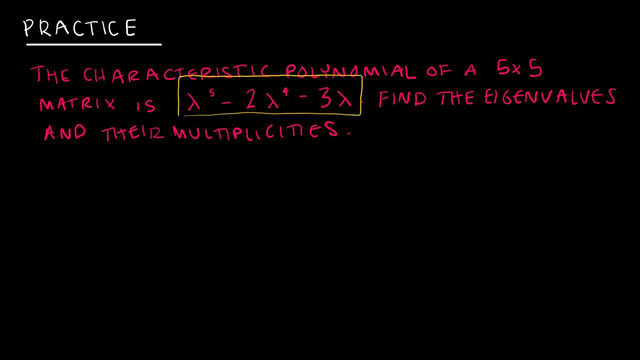 which is lambda to the 5th, minus 2 lambda to the 4th, minus 3 lambda to the 3rd. We are asked to find the eigenvalues and their multiplicities. So they've given me the characteristics. So this is a characteristic equation which is just the determinant of the 5 by 5 matrix. 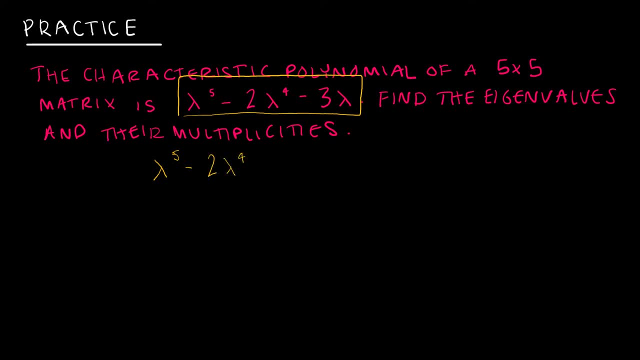 and it's lambda to the 5th minus 2, lambda to the 4th minus 3 lambda to the 3rd. If you'll recall, we just set the equal to 0.. We set the determinant equal to 0.. 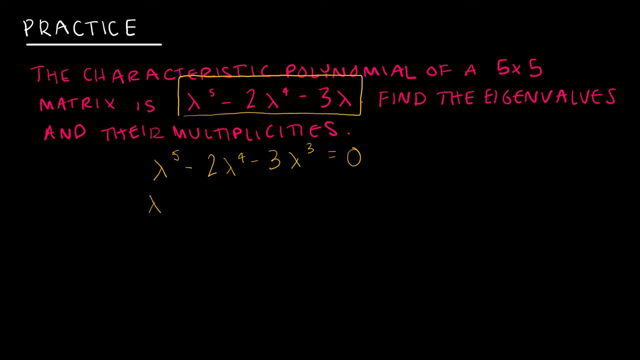 From here. this is just algebra. So this is lambda cubed factored out of each, and that gives me lambda squared minus 2. lambda minus 3 equals 0.. And then lambda cubed, and then I'm just going to factor that trinomial. 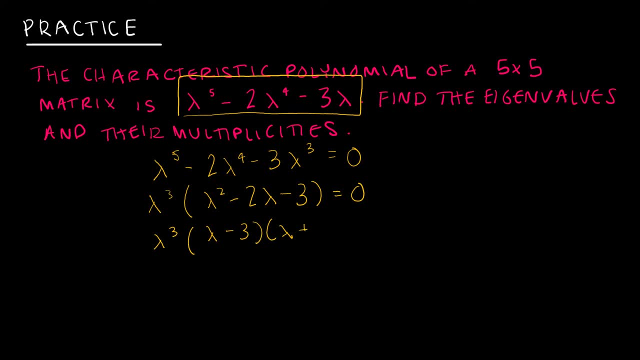 So lambda minus 3, lambda plus 1.. And so again, this is my characteristic polynomial, just in factored form. I'm to find the eigenvalues and their multiplicities. So I'm just going to take each of the factors and set it equal to 0.. 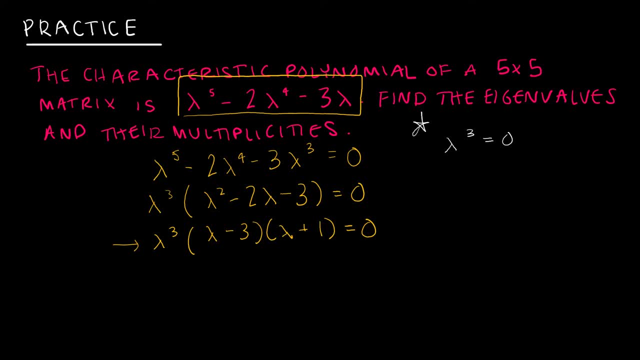 And no, you do not need to show all of this, I'm just showing you, just in case You've forgotten how to find the zeros of a polynomial. We're going to take each factor, set it equal to 0. So I have an eigenvalue of 0, and this was 3 times. 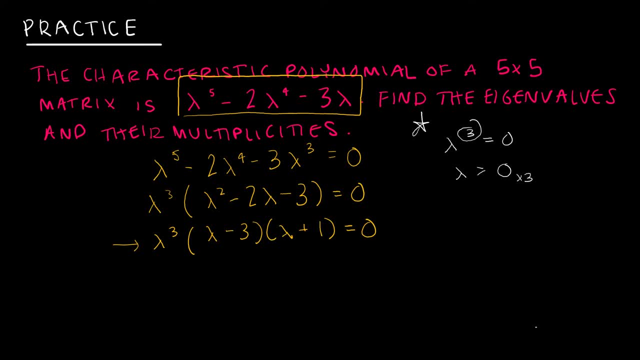 So this actually has a multiplicity of 3.. And then, of course, I would take: lambda minus 3 equals 0. So lambda is equal to 3.. And then lambda plus 1 is equal to 0..